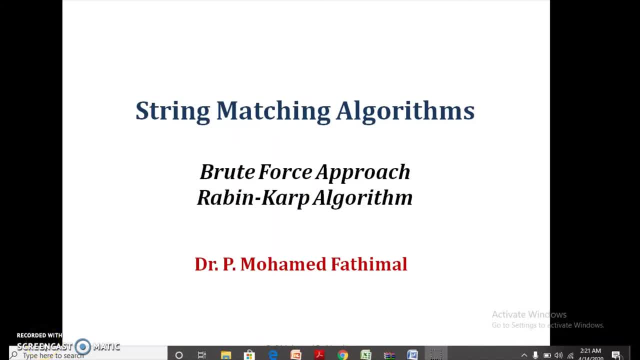 Hi, in this video we are going to study about string matching algorithms. I am discussing two algorithms. One is Brute force approach and another one is Rabin-Karp algorithm. So for brute force approach, naive pattern matching algorithm is discussed here. 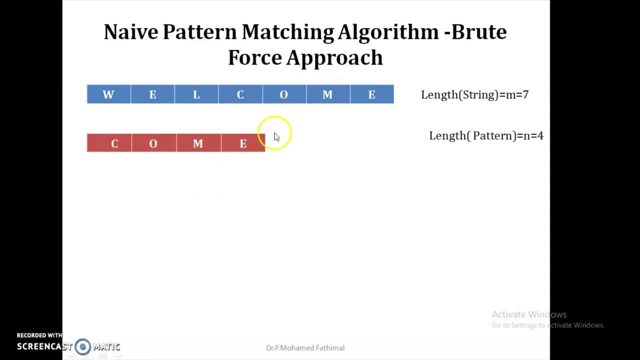 The objective is will be given with a text and a pattern and we have to check whether the pattern is available in the string or not. So for this, this complete text will be taken and it will be divided into substring of size same as the size of the pattern and each characters of the pattern. 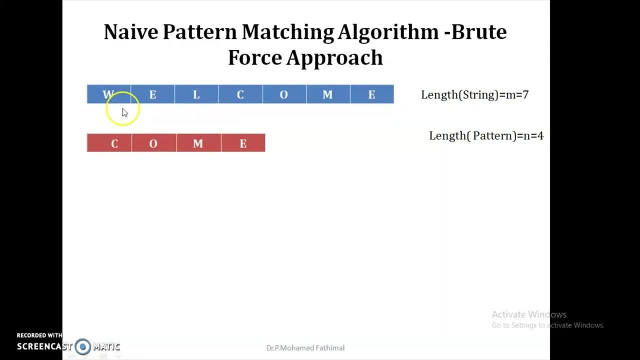 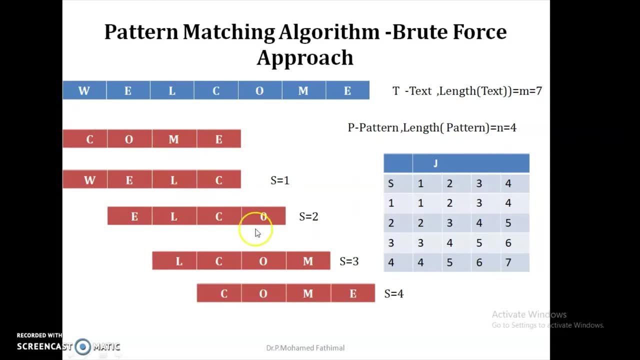 will be matched with the patterns of the, the characters of the substring Right. Let's see that here I am dividing this complete text into substrings like this. First time I am taking welc the first four characters, as the size of the pattern is four. We are taking first 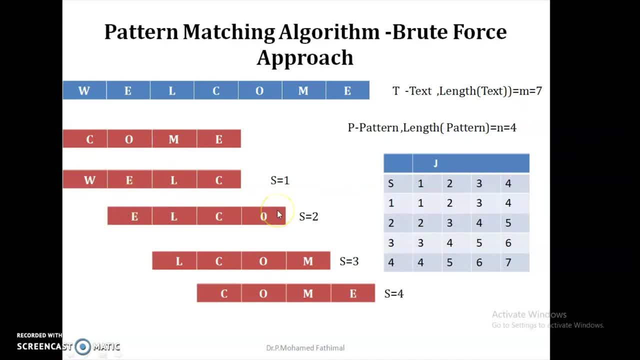 four characters. Second shift, I have taken from two to five and for the third shift, i have taken the characters from three to six and for the fourth shift, fourth to seventh character. so this in this chart i have given what is the total number of shifts required. 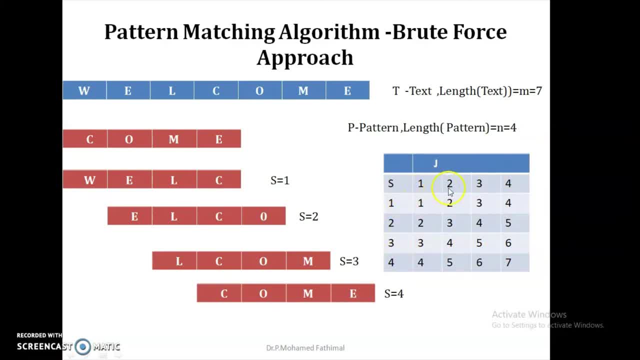 and then here this column refers number of characters in the given pattern. so the first character of the pattern is matched with first character of the text in the first shift, right? if they both are equal, then it will proceed and checking the remaining characters of the substring. if it is not matching, then you will skip this and come to the second shift. 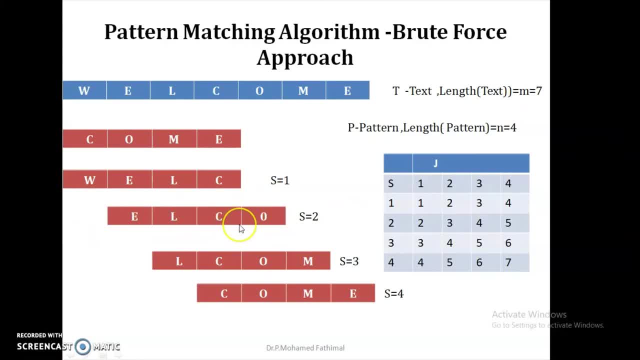 now we are going to take the second substring of the given text. now the first character of the second second substring is compared with c. so that's what given here. the second character of the string is compared with first character of the given pattern. so if they both, 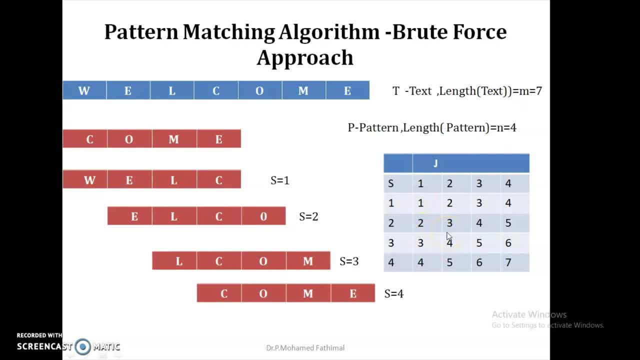 are same, then it will start proceeding with the matching checking the remaining characters of the substring. if it is not equal here, in this condition, here c is not equivalent to e, so it will skip. it will come to the third shift. in the third shift it will take the 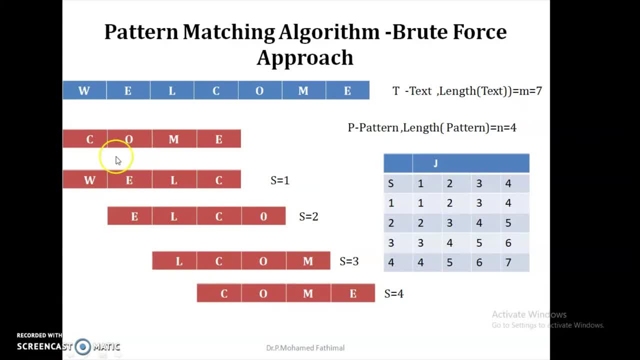 characters from the third position and the third character of the text is matching with the first character of the pattern. they are not equal, so come to the fourth one. now here, the fourth character of the text: Почему它ає TRATIη terme? 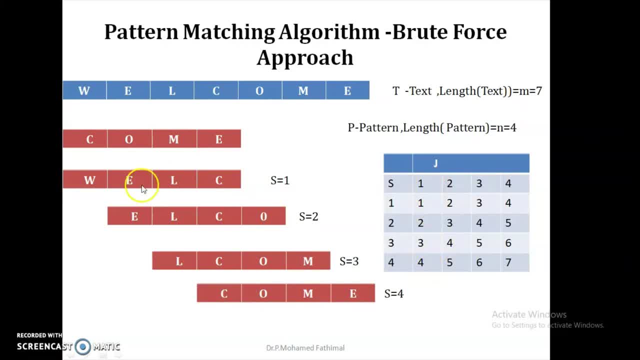 ahan is taken and now it is compared with first character of the pattern. they both are same. now it comes to the second one. a next one, that is, first character of the given text is compared with second character of the pattern. next third with 6, as they both are equal. 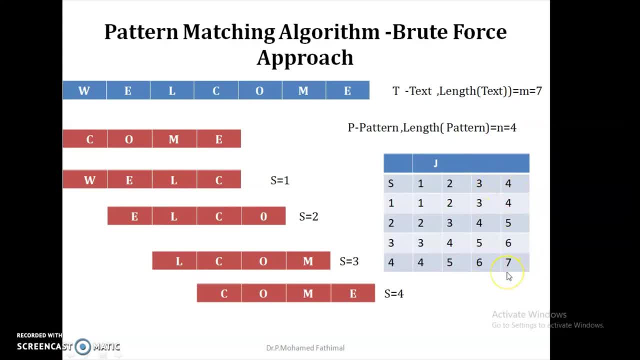 next, fourth character of the pattern is compared with seventh character of the text, so they are equal. so at this point we can tell that the pattern is available in the given text and the position is fourth position. right, so lets write algorithm for this. just let us take this chart every time. 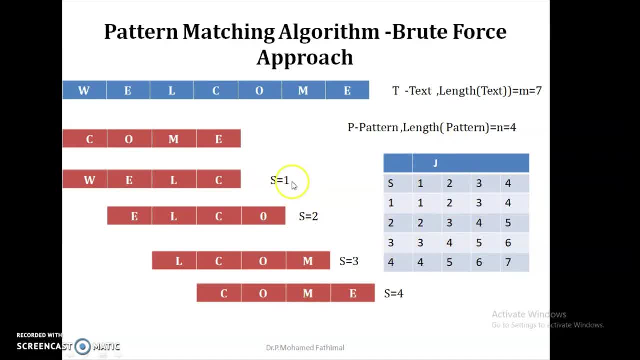 how many shifts we have taken here. totally four shifts. this number of shifts is based on the length of the text and the length of the pattern. so length of the text is 7 minus 4 plus 1. that is equivalent to the number of shifts here and in each of the shifts we are. 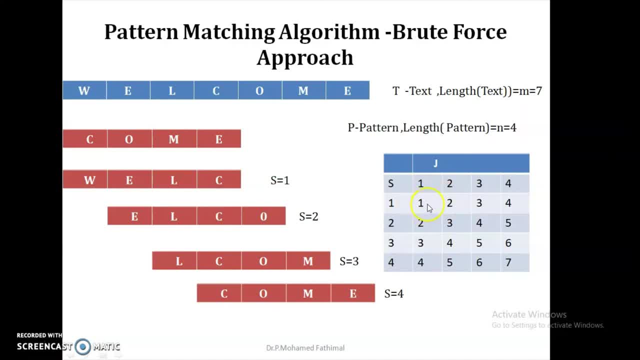 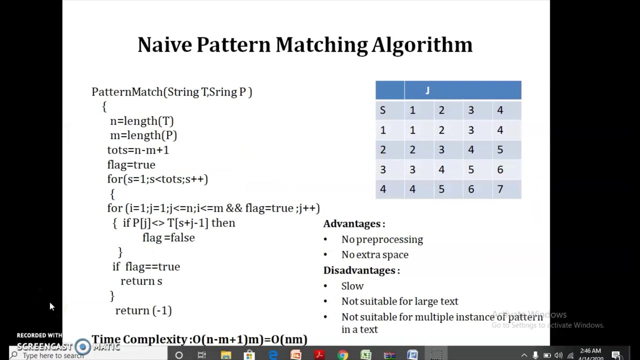 comparing the given pattern with the text of the Avidya text. right, so the position of the text is given in these cells. so what is the relationship between this position and the shift and the pattern position? right so J plus S minus one. is this one: one plus one minus one. one plus two minus one, the name pattern. 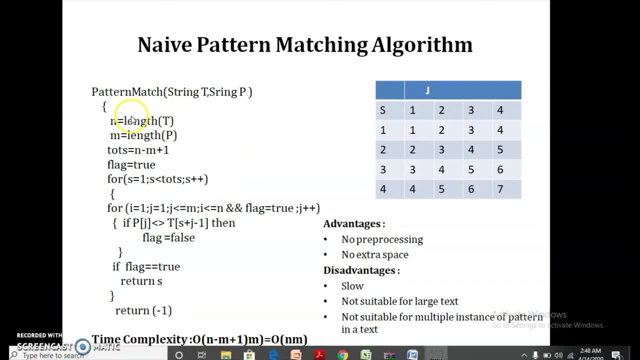 matching algorithm is given. so initially we are finding the length of the string and the length of the pattern and the total number of shift is n minus n plus one, and set the flag as true. this process is repeated for total number of shift times. initially, the condition for the i and j values are telling the one. 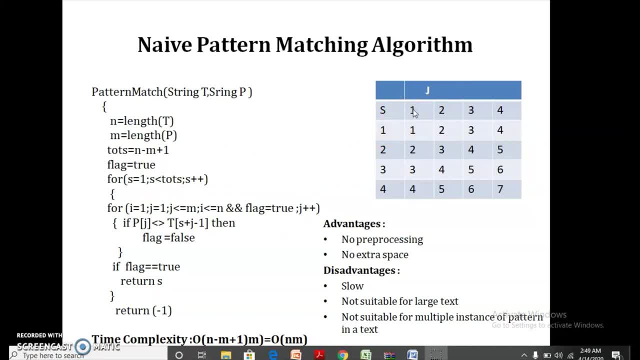 one or nine. one, that means we are checking the first character of the pattern with the first character of the string. so both are one and we are repeating this process until i, j reaches the fourth, that is, the length of the pattern, or i reaches the seventh position, right, so that is n here. 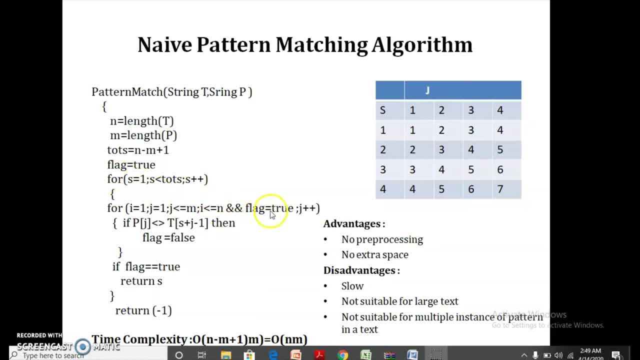 and where the flag should be always remains true. when will the flag becomes false is if the character in the pattern is not equivalent to character in the text. that time the flag becomes false and we can skip the process. remaining character matching will be stopped at that point. 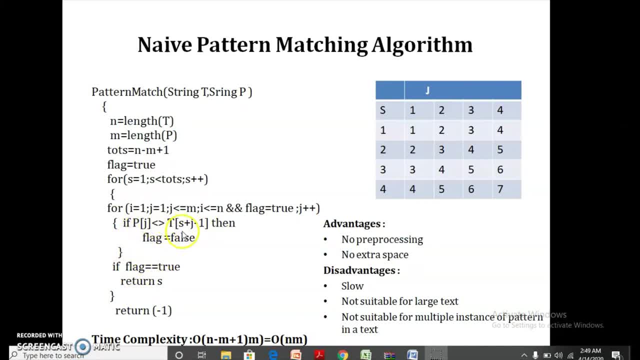 so all the characters are matched, then the flag will remains as true and we can return the position of the particular pattern in the text. otherwise, if you are repeating all these process and you cannot get the final character means, then you can return it as minus one. so what is the total time complexity for? 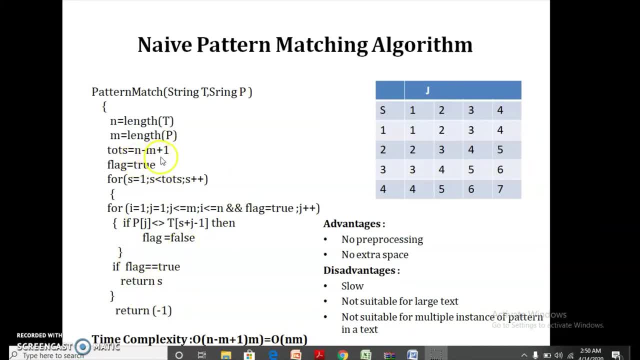 this, as we are repeating this for n minus m plus one time. so we go off: n minus n plus one is given, and that should be in each and everything. we are having m number of comparisons. so if the length of the text is very high, then n. 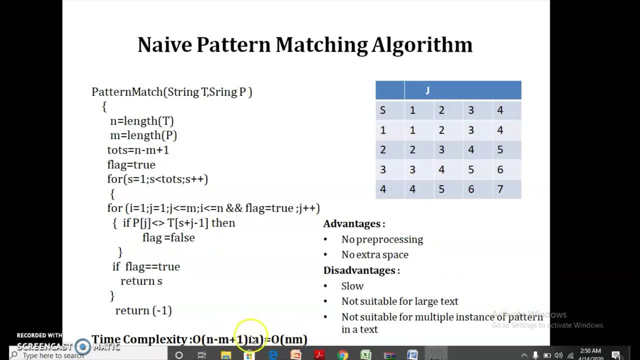 will be very high when comparing to m. so we are taking the total time complexity. the worst case is we go off n. so what is the advantage of this name pattern matching algorithm is it doesn't need any pre-processing and it doesn't need any extra space. but it is very slow and in the case if the pattern is occurring, 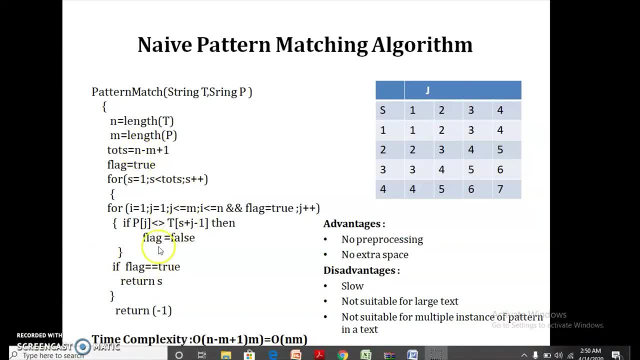 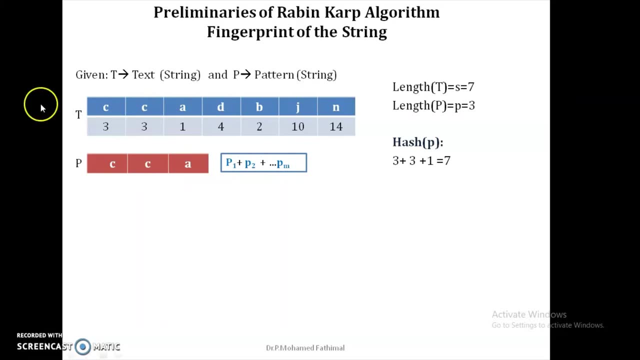 for more than once. this algorithm will not help you to find the number of occurrence of the particular pattern. so we are going for Rabin Karpal guard. so what is Rabin Karpal guard? instead of comparing each and every character of the pattern with the character of the substring, here we are. 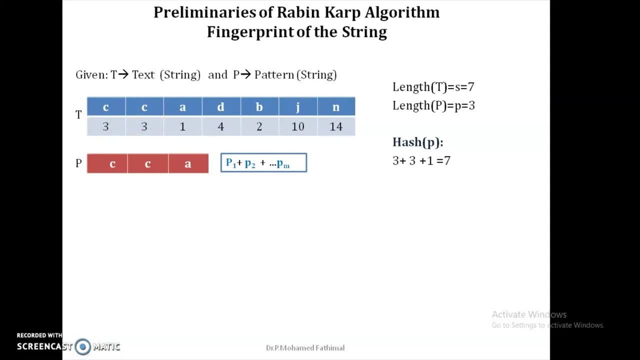 going to find hash of the substring and the hash of the pattern, so let's start with that for better understanding. let us start with finding the hash for the pattern using simple hashing algorithm. right, the objective is same here. also, we are going to divide the text in two substrings and then we are 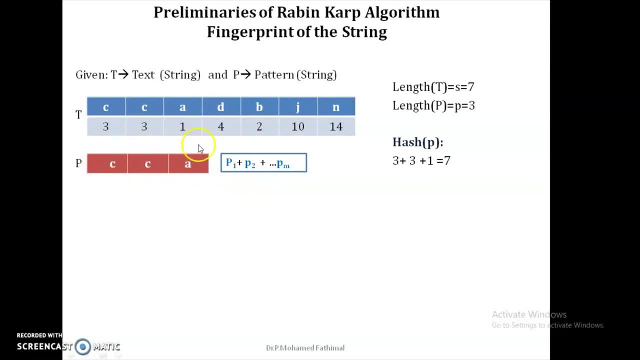 comparing the hash value of the pattern with the hash value of the substring. let's see here the example is given here. the example is example: text is CCAVBJN and the pattern is CCA and instead of comparing character by character, we are going to assign some. 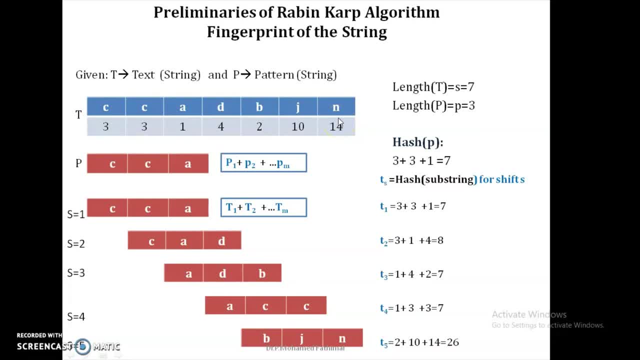 numeral for this, each and every character. so let's maintain one hash table and if we are using 1B alphabets we can take the numbers. ordinal position of the alphabets. a is 1B equal to 2, like that, and we can have it in a hash. 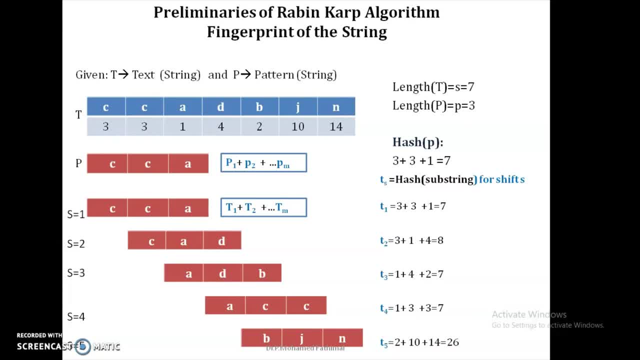 table or in case, if you want to use ASCII values, you can use that also, and the corresponding hash values are given here and now we are going to help calculate hash for the pattern as well as hash for each of the substring. so the simple hashing is this: we are going to add the values of each and every character in. 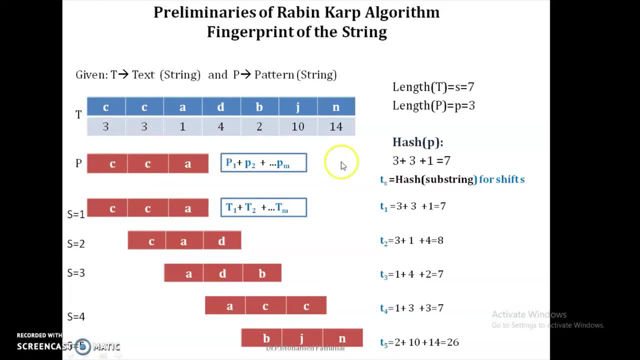 the substring. so pattern for the pattern: the hash is C is 3, right 3 plus 3 plus 1, 7, and for each of the substring first character for substring is CCA, so here also 7, and here we are having CAB, so the 3 plus 1. 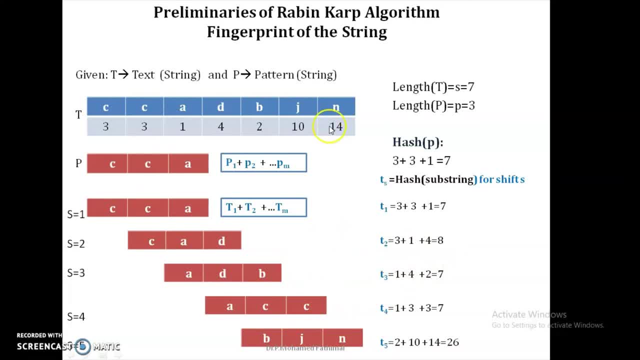 plus 4, equal to 8. likewise you are doing here. so but what is the length of the string here? length of this string is 7. what is the length of the pattern? only 3, right. so 7 minus 3 plus 1. 5 shifts are here in the 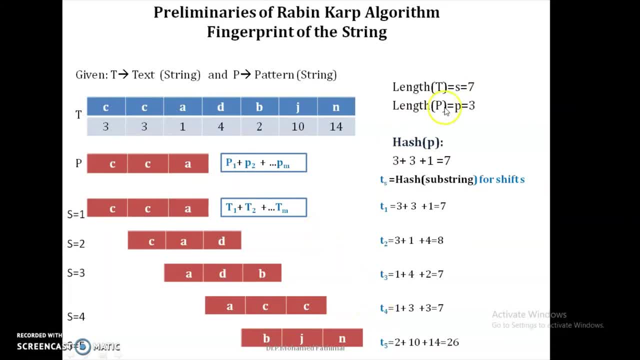 previous example, you have seen only 4 shift, as the length of the pattern is 4, but here the length of the pattern is 3, so we are taking this as your number of shifts, right? so instead of doing comparisons- m- number of comparisons- we are just doing m- number of subtractions, right? so we are 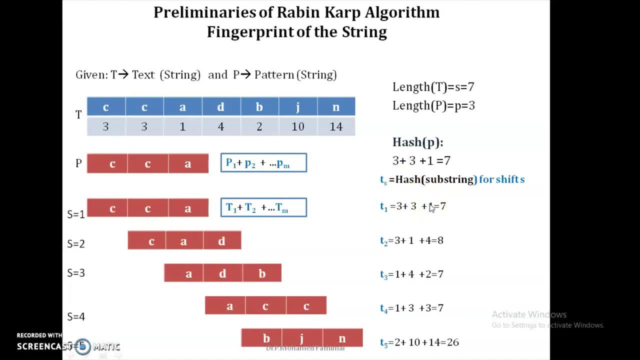 comparing the hash values. if you are taking the hash value of the t1, this is equal to this one, the pattern of the patterns, hash. so we can take this as a value shift. okay, and if you are taking the second one, the hash values are not same. and if you are taking the third one, the hash values. 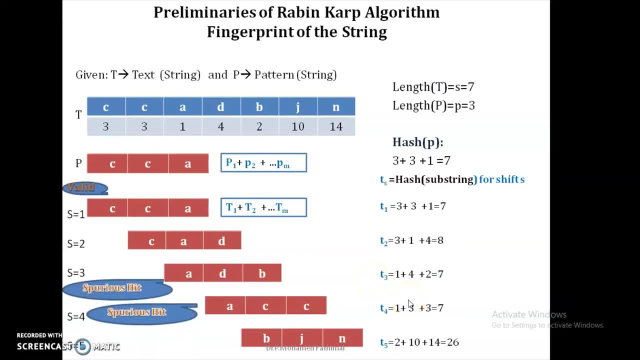 are same. and fourth one is also: hash values are same. right so. but if you are comparing the characters of the first, shift the characters one by one. we have to compare with pattern. so we are taking the second one, the hash values are not same. and if you are taking the third one, 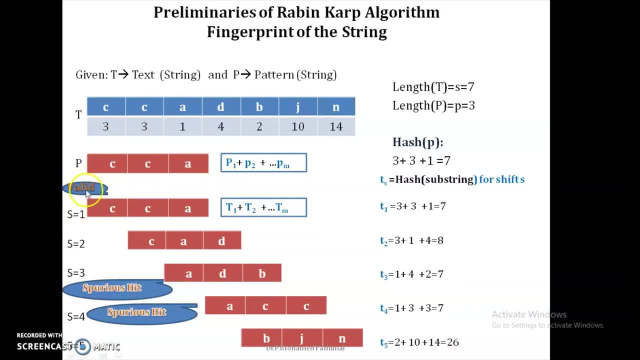 they are all same. so this is a valid pattern and valid shift. but when you are taking this third shift and fourth shift, when you are comparing the characters, even though the hash values are same with the hash of the pattern, but the characters present in this are not equal. so 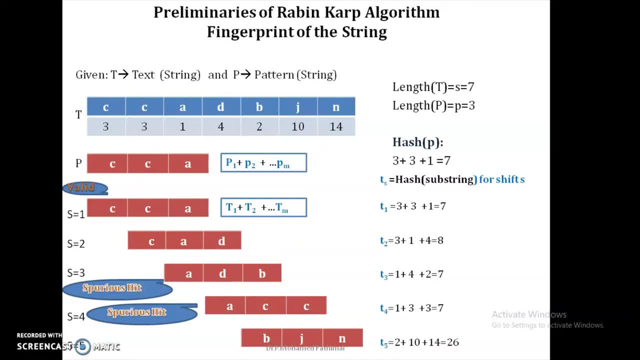 what you have to do is in this Rabin-Karp algorithm, in the stage one, we have to find the hash and compare the hash with the hash of the pattern. if they are same, then once again we have to do brute force approach to compare the particular substring with the pattern. okay, so 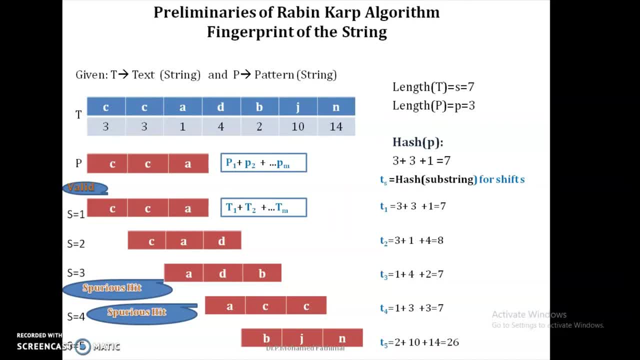 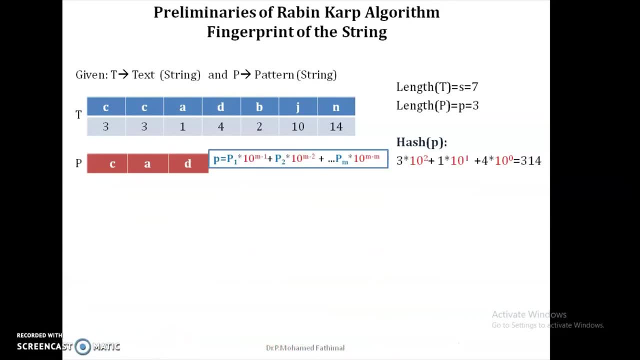 our objective is to reduce the number of spurious heat. so in that this is a spurious heat, we have to reduce it. let's take one more hashing algorithm. as the number of spurious heat is more for the previous simple hash value, we are going for the next level. here we are assigning some decimal. 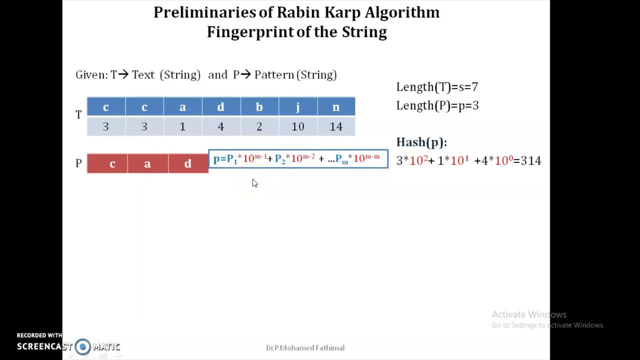 value as the base, as the number of spurious heat is more for the previous simple hash value. we are going for the next level. here we are assigning some decimal value. we are going for the next level as we are using the base decimal values. here we are taking bases 10 for simplicity and we are 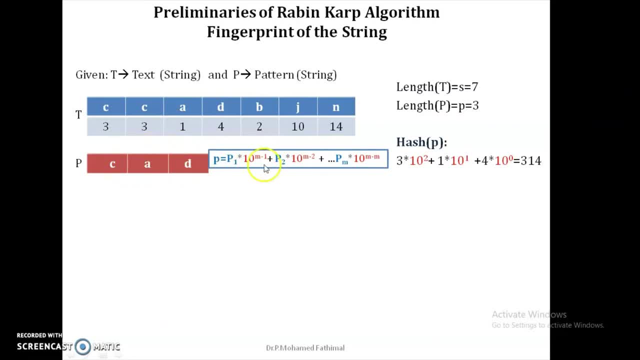 calculating hash like this: each digit is multiplied with the value. of this digit is multiplied with the base to the power m minus one. so for the pattern we are having, 3 into 10 to the 10 square plus one into one is for a 1 into ten to the power 1 plus this one is four into 10 to the power zero. 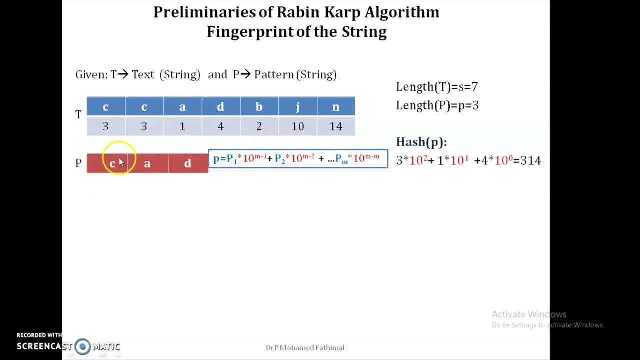 That means zero is position first position, second position, second position and third position. first second question: like that, zeros, tens and hundreds in there, okay, so similarly, we are going to calculate the same hash value for each of the substring and we are getting the values like this: for the first substring: we are getting 3 into 10 square 300 plus 30 plus 1 right and 10. 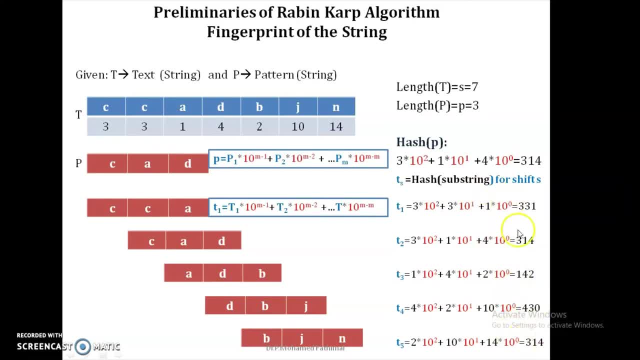 to the power. 0 is normally 1, so we can skip this part. we can reduce this code also. and here, what is the value of t1, t2 and all? so what is the hash value here? 314. but here, in this substring, we are getting the values of the 314 in t, s2. that is, this cad, as well as in the last one. 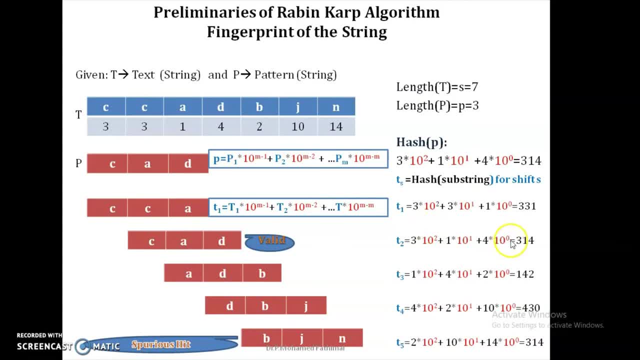 but if you are taking this one, as the hash value of this t2 is equal to the patterns hash value, now we have to check character by character. c is the first character of the shift and c is the last character of the shift. and c is the last character of the shift. 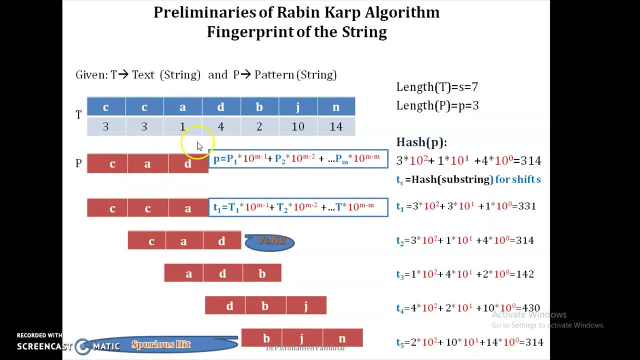 and here also c and a and d say they are same. so this is a valid shift. but when you are taking this fifth shift, first character is b, but here the first character is c. they are not these two. this pattern and the substring is not matching. but even though the hash values remain same. 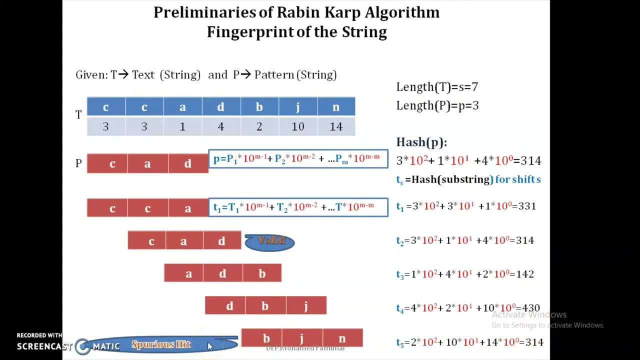 so this is curious here. so we have to reduce it again and also we have to check: is there any possibility to reduce this calculation? let's take the calculation of t1 and t2. here c is the calculation for c and a, and c and a remains same for both the t1 and t2, but the position 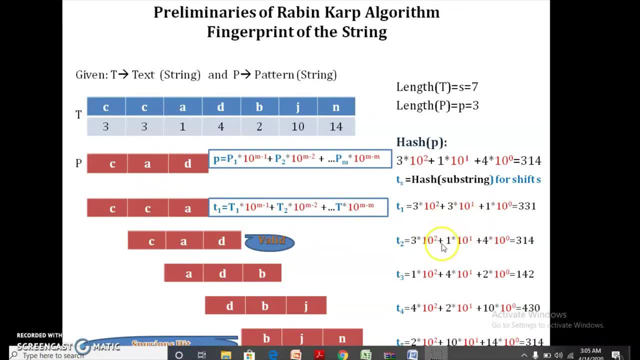 is left shifted by once. so just, we are multiplying it by 10 here. so 3 into 10, square 10 is 30 becomes 300 and 10 becomes- and um sorry- 1 becomes 10 here. so let's try to calculate. uh, only uh, these two. 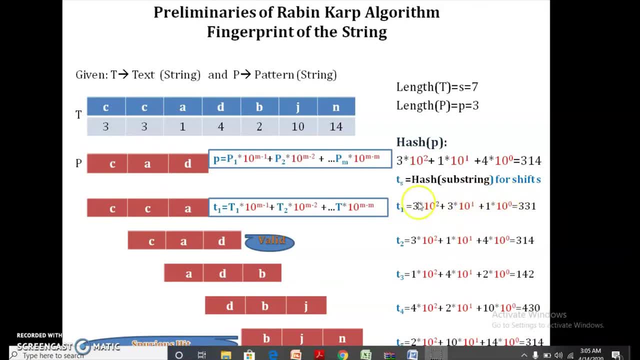 terms by subtracting this t1, mine uh, from this, is this the first term, right? so let's take, instead of having this, we are going to uh multiply 10 by this term. this term is nothing but t1 minus 3 into 10 square. let's see this here. 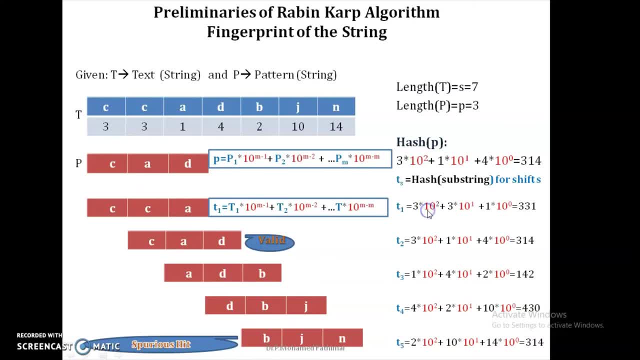 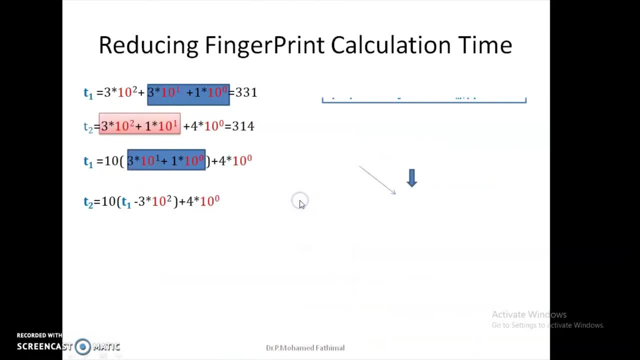 here: t1 is this one and t2 is this term, and instead of having this, we can just take 10. now we are getting these terms same as this one, so this can be replaced by t1 minus 3 into 10 square. so that is replaced here as t1 minus 3 into 10 square plus 4. 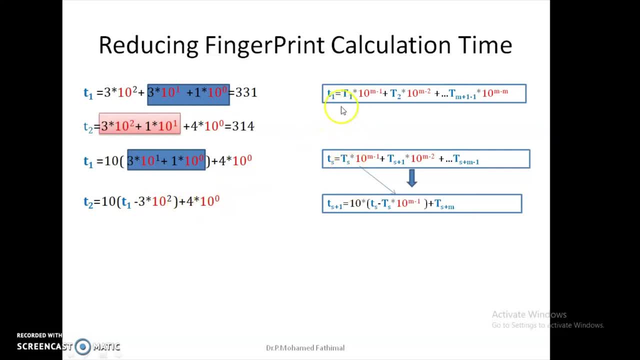 into 10 to the power 0.. when you generalize this, uh, initial first substring should be calculated as such. but when you are coming to the second and successive, all these shifts, we are calculating based on the previous value. what is the previous value? previous value is: 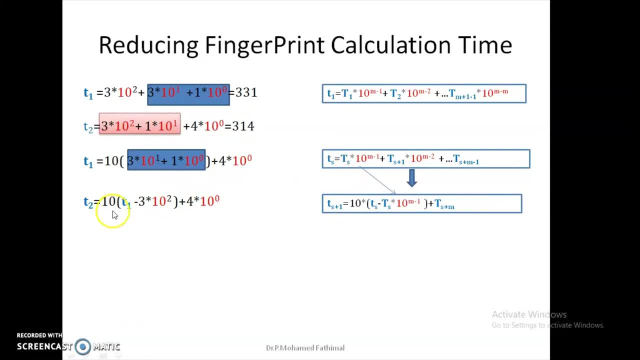 we are multiplying right. so our 10 into t s is the previous value, right. if you want to calculate t2 we have to take t1 value right. t s minus this one is 3 is from the first position of the t1 right. so here the previous shift, first position will be taken here this one t s minus t s into 10 to the. 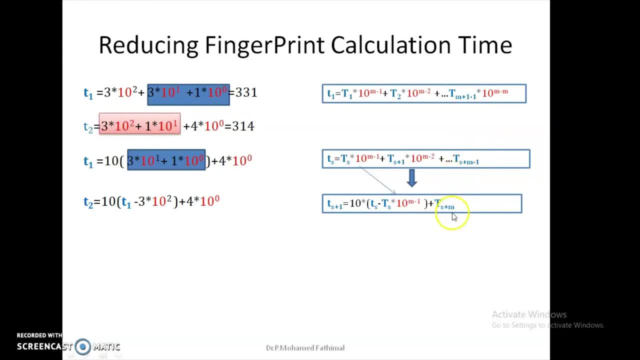 power minus 1 will be taken plus the last one is t s plus some for this right. so this is what we are going to do. so, instead of having m number of multiplications and m number of additions, we are reducing it by having, uh, all the m minus 1 number of subtractions will be a multiplications. 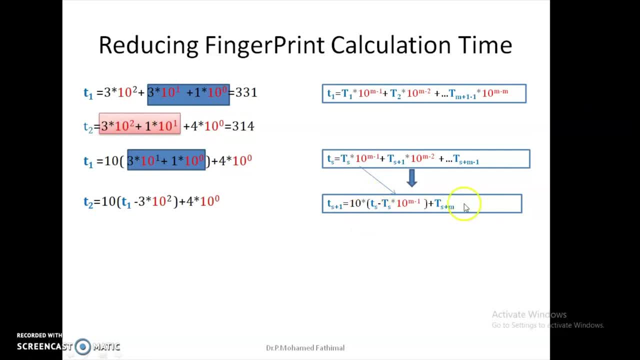 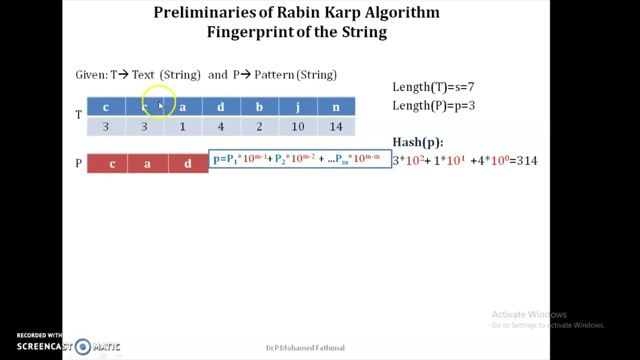 will be reduced and you will be having only single multiplications and only one addition here. one addition and one subtraction will be here. so this is a one way to reduce the fingerprint calculation. let's see the same example here. initially we are calculating the first text as the previous calculation, and also the first text is also calculated. 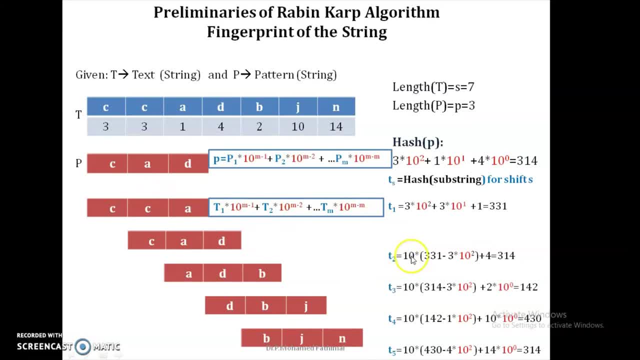 and now, if you want to calculate t2, i'm just taking 10 into 331 minus 300, right, this term minus 300 plus the. what is the fourth character? uh, fourth character is d. so, uh, fourth character is d, so its value is four. so 331 minus 331 into 10, 310 plus 4, that is 340 here. 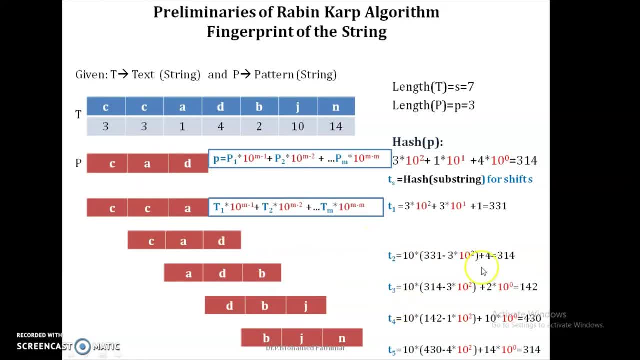 when you are taking p3. this a, d remains same. no, so we are taking: uh, just going to subtract this value, this value into 10 to the power square right, so 314 minus 300, plus what is the value of b 2? 2 into 10 to the power 0,000, so 142. if you're taking t4. 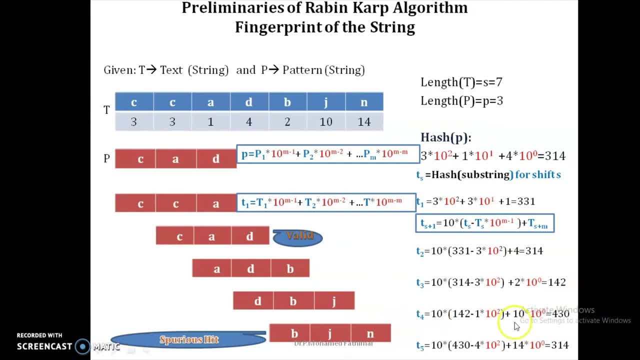 d and b remains same, just you have to take this into 324, t4 is 430 and t5 is 314, t5 is 314, t5 is 314, so in t6, t6 is 434, t5. we are subtracting the left out character d, so 4, into 10 square and adding the new character. 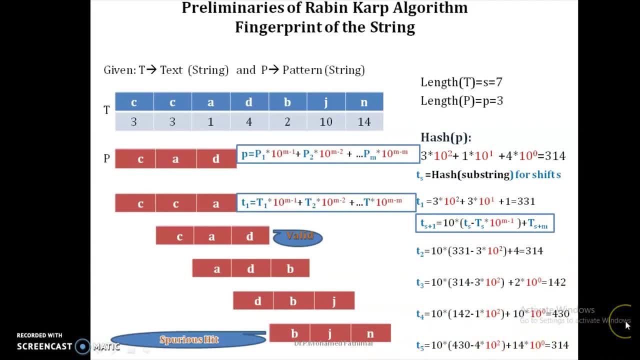 n, which is whose value is 14. so we are getting the value as 314. so out of all the hash values available for all these substrings, t2 and t5 are producing the same hash as that of the hash of the pattern. but let's see whether the pattern is same. so if you are taking t2 again we have to go to. 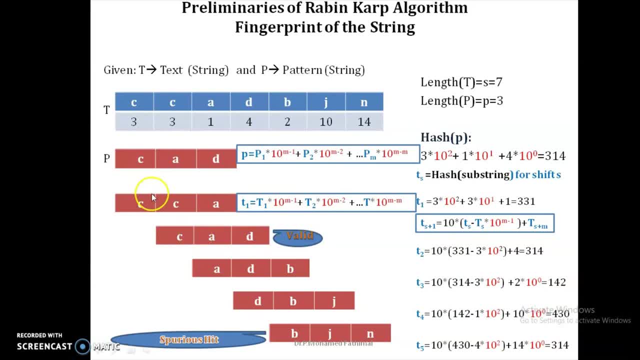 brute force approach and check character by character. here the characters are cad and here also cad, so this is a valid one. but when you are taking this t5, even though the hash remains same, the characters are not equal, so this is a spurious hit. okay, so if the number of characters are more? 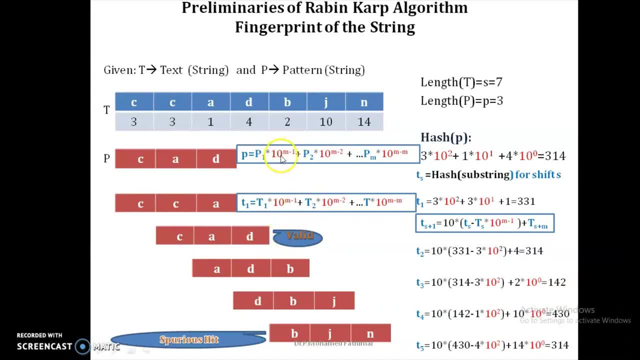 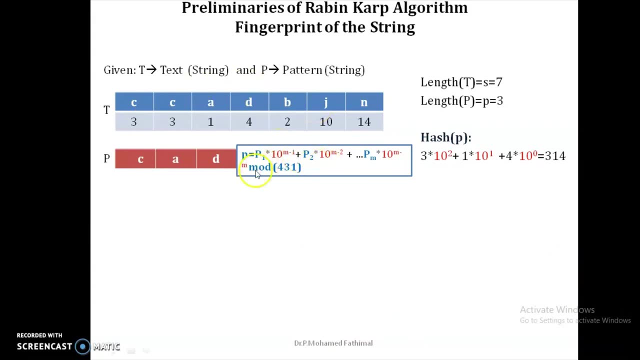 in the hash table. and if you are taking the decimal values instead of this base as 10, if you are taking a larger value, again the calculation is getting inaccurate. calculation will be more complex. so for that we are going to a modulo arithmetic. so instead of normal multiplication and subtractions we are taking going to take the mod of 431. so where? 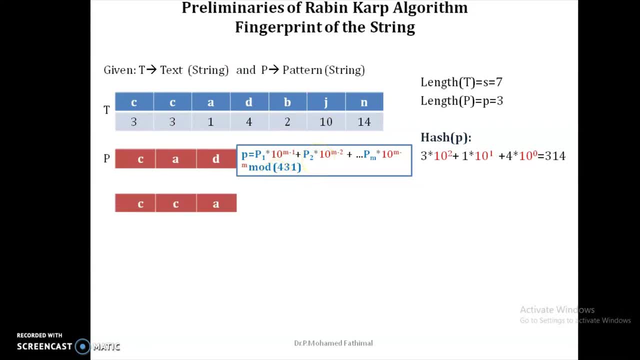 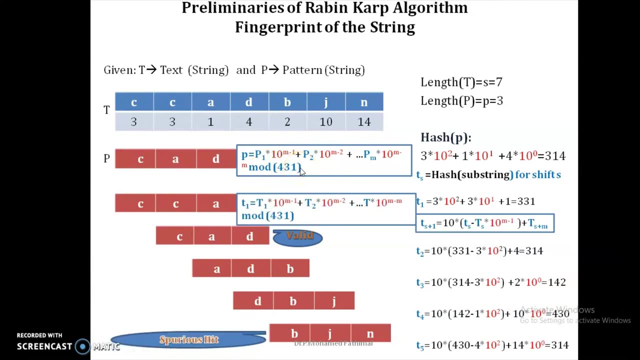 431 is the prime number i have taken here, and then, in the same example, i am getting these values: 3, 14, 3, 31, and on all these are lesser than 431, so there is no change in this value. to understand this usage of this modulo arithmetic, let me take one more example. 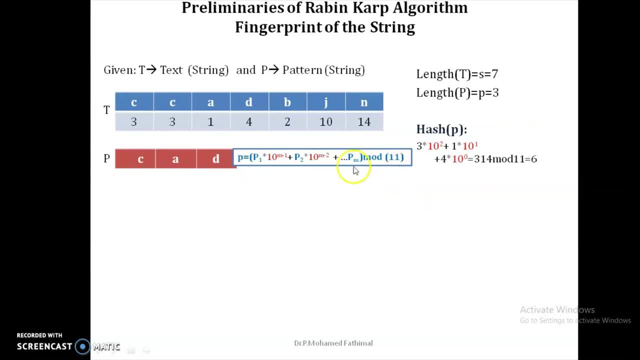 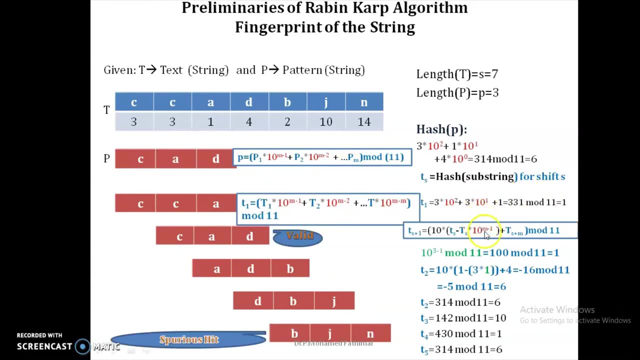 here i am taking the prime value as 11. so if you are calculating this, 3 14 mod 11, it will become 6. so the number is getting reduced and it is very easy to calculate too. so for the text also, when you are doing this, in each of the we have to calculate 10 to the power minus 1. so let's do. 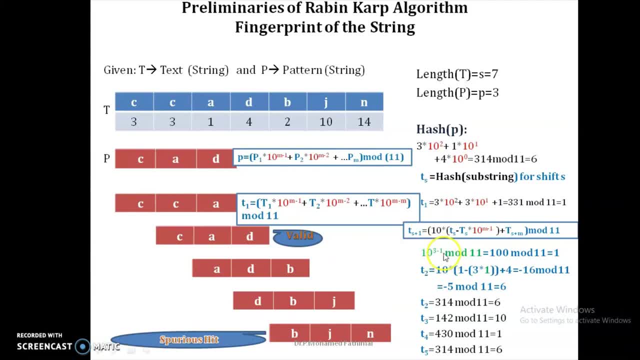 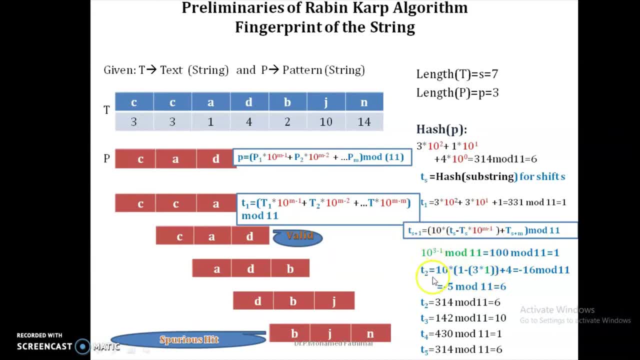 this: this is replaced by 1 here. so if you are taking t2, 10 into t1 is 1 in minus t s is that is t1 is 3 into this 1. uh plus 4, that is minus 6 mod 11, so it is 6. so for t2 also, we are getting like. 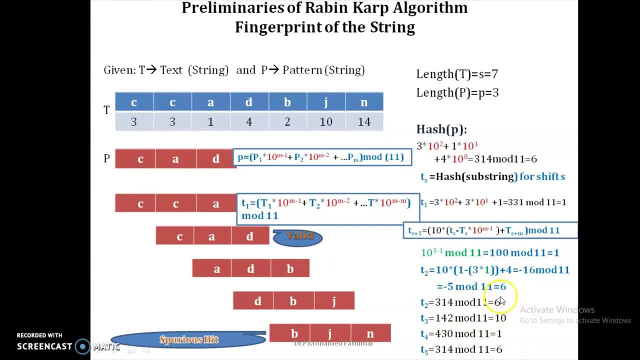 this t3, t4 and t5, so the number of spurious hits now is a number of matching hash values are t2 and t5, but t2 is- uh, you are taking t2. the characters are same as the pattern, so it is a value shift. but 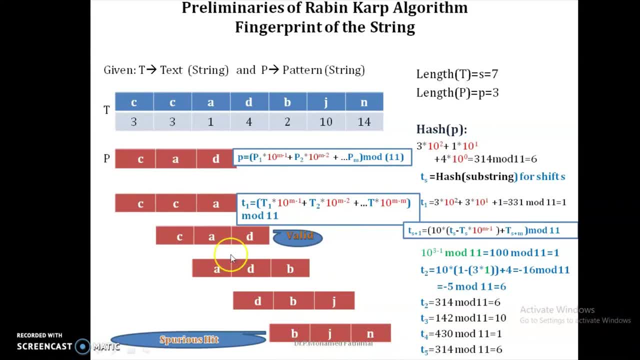 when you are taking the t5, the characters are not same as the pattern, so it is a spurious hit. so let's write the algorithm for this. let's summarize what are the things we have done. if you are taking, you were given with the text and the pattern, we have to find the length of the 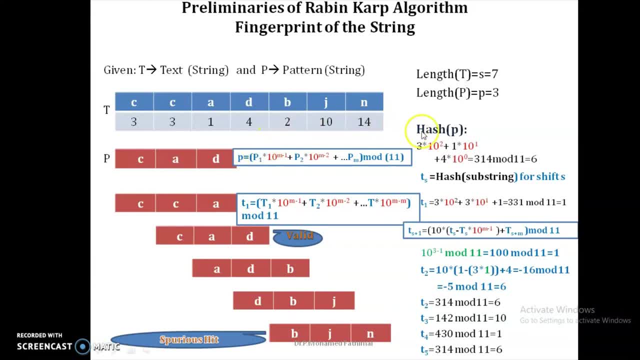 text and the length of the pattern and find the hash value for the pattern as well as for the first substrate. so for this we need to do a separate procedure and for the successive hash value, uh, for the successive uh substrings, we have to calculate based on the different formula that is in a 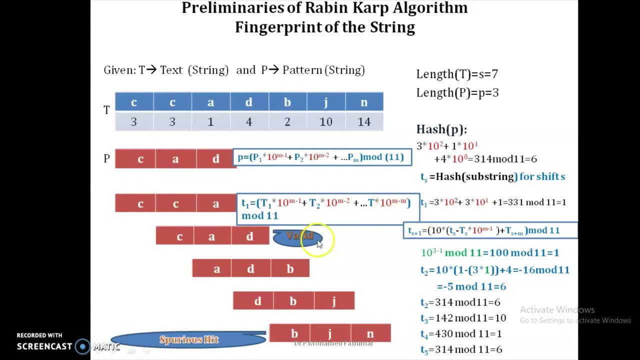 separate loop. so every time we have to check whether that hash value is same. if the hash value is same, then we have to compare character by character. that's what we will see in this algorithm. i mean cup matcher algorithm, and given text is t, pattern, p, decimal. 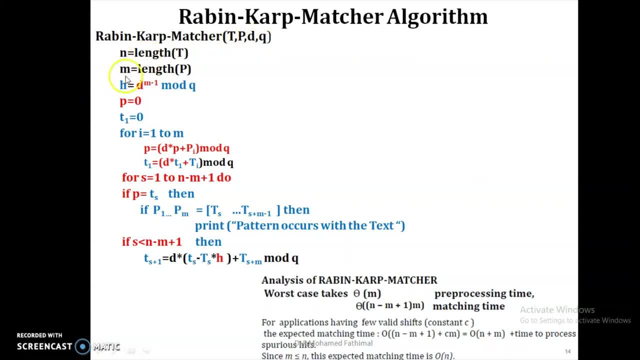 d n prime key. first find the length of the text, n length of the patent, n find the hash value, which is due to the code m minus 1 mod 2, which is common for all the successive text, and to calculate the initial um substrate hash, as well as for the pattern, we are uh having two initial 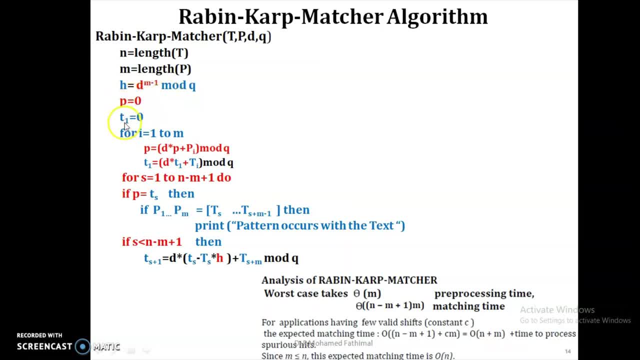 variables. p is for hash value for uh pattern and t1 is the hash value for the first substrate, and we are calculating this p as each time we are calculating the initial bound and the final bound has the punished hash. as you have calculated, t1 is the hash value for this and we have to. 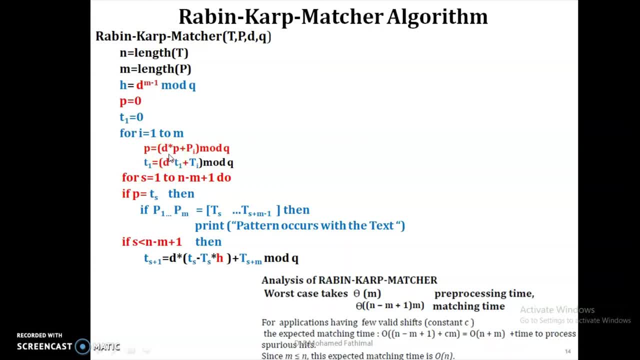 start with the variance. so here it will be. the finished pattern is the hash value, which is divided by two, just like this, and throughout the field of output, so that we cannot calculate the Awesome- and taking the particular character hash value and multiplied by decimal value and the successive. 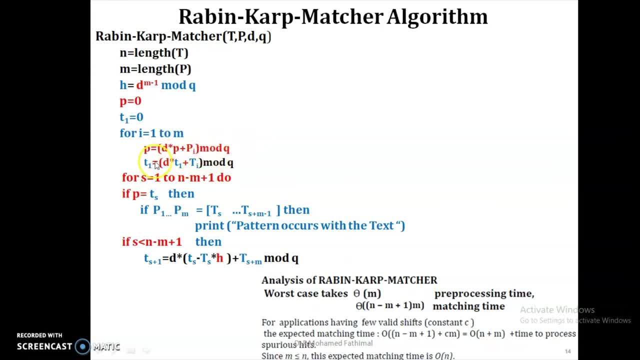 characters are added and find the mod of it right. so d into 10, for example, 10 into 0 plus first msb position will take mod q and second time this is the msb is multiplied by 10 and the second digit. so likewise you are calculating the same way for. 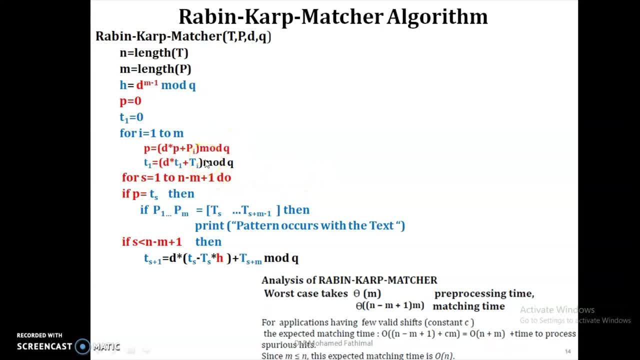 text substring of the first substring also. so the hash value of the first substring is t1, hash value of the pattern is p, and now we are checking whether they both are same. if it is same, we can write. the pattern occurs within the text and also we will not stop here. 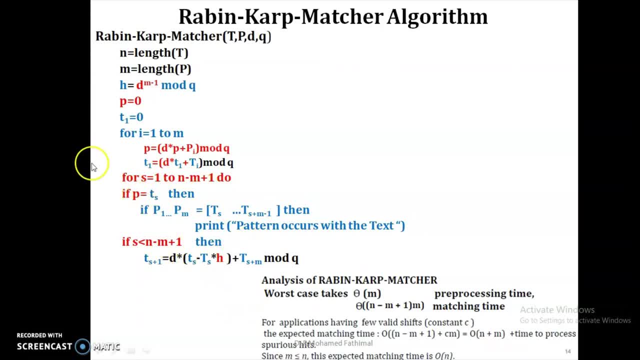 we have to see for all the successive characters, and so that's why we are having this loop. in this loop we are taking the shift from 1 to n minus m plus 1 loop, the. so for number of shifts. we have already discussed, so same thing we are using here. 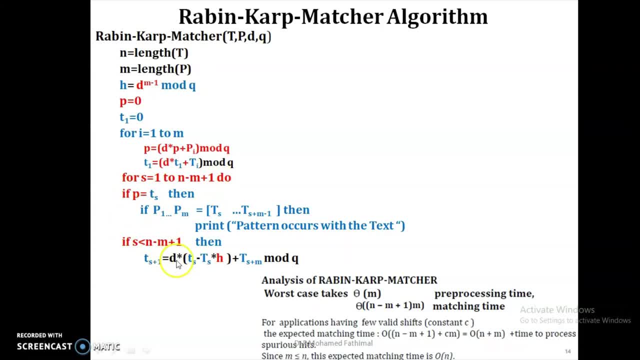 if, until you reach this shift value, we have to calculate the successive hash value as the decimal value into the previous hash value minus the left root character, into h, h is d to the power m minus 1, the most significant digit. we have to subtract now so that value plus new coming character, mod q. so this is what. 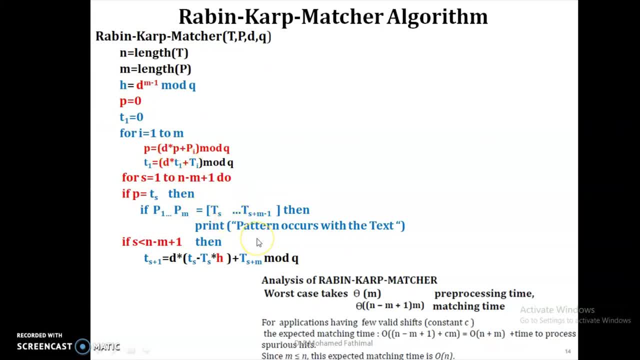 you want to see after we have taken those two discriminations. you have to also do that. we can write this value down and we can see that in this little next quark you can see your group four itself, given that group three has done a solution v, as well, as if they are appear. so 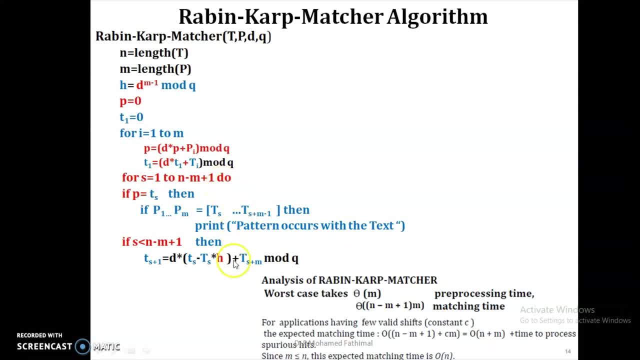 we can put the final Imaginal positive argument in each group before we divide by n. maybe we just get the top element. we willcks the next left root. so it's a t2 is not aragis. totally. you will be having n minus m plus 1 into m matching time but practically number of 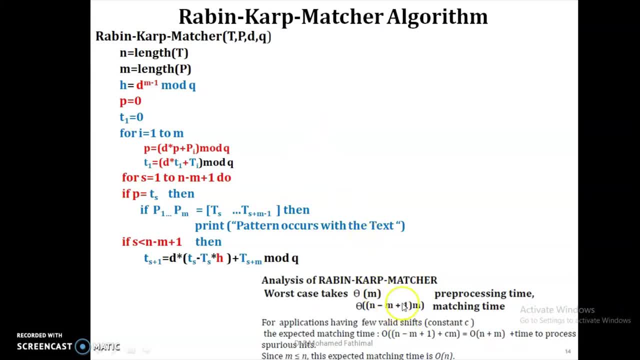 characters in the text will be very large when comparing to number of characters in the pattern. so we can reduce this or we can neglect this. m plus 1, so you will get order of n and this one is. m is a matching time, so if you are having very less shift means this will not be m and it will. 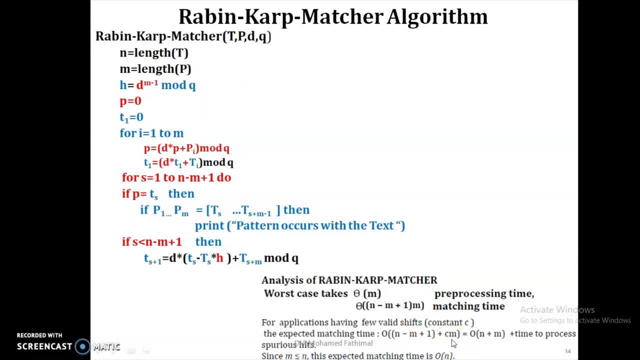 be taking some c value only. say right, so we are taking order of n minus m plus 1 number of calculations, that is, this hash calculations plus cm is for time to take an valid shift. that group force approach plus time taken to process here, curiously. okay, so we are taking n only here as.